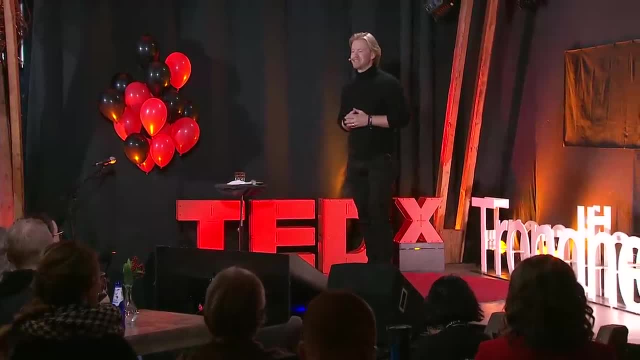 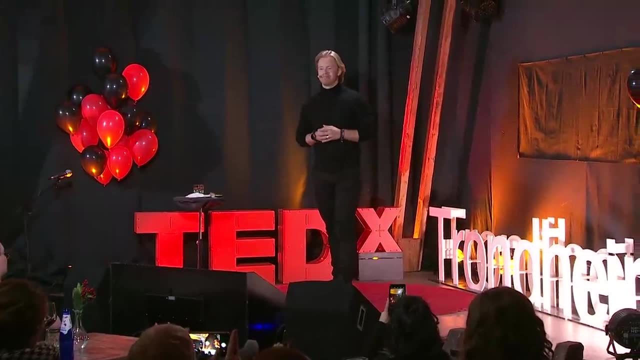 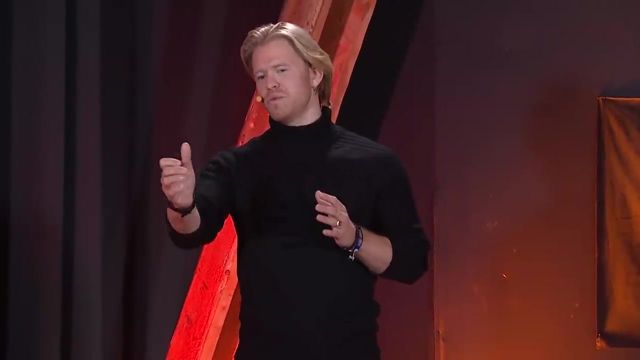 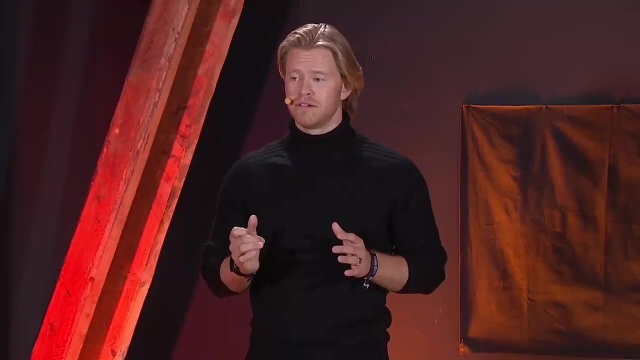 Then we have human-machine interaction, and that occurs when we as humans want to interact with or control any kind of machine- and that's what I'm going to focus on here today- Like when you want to pull a lever to control a crane. if the interaction is designed well and you know what to do, it usually goes right. 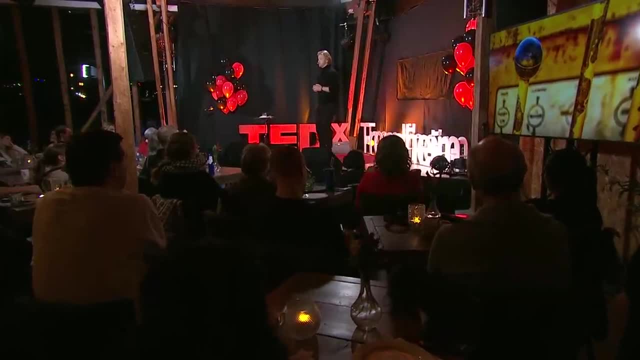 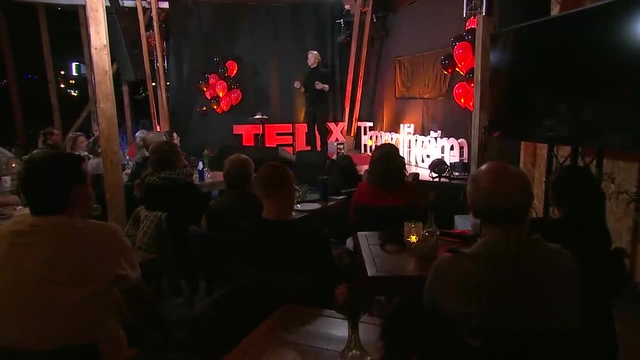 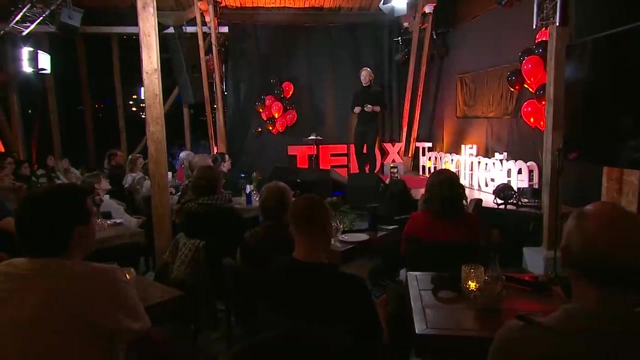 But this requires Some sort of Afterthought, training or practice. A hundred years ago, machines were mostly mechanical in their nature and they were built in such a way that they require a very specific set of input actions in order to work as intended. 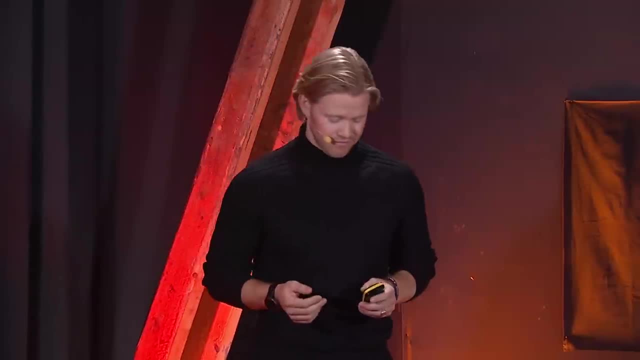 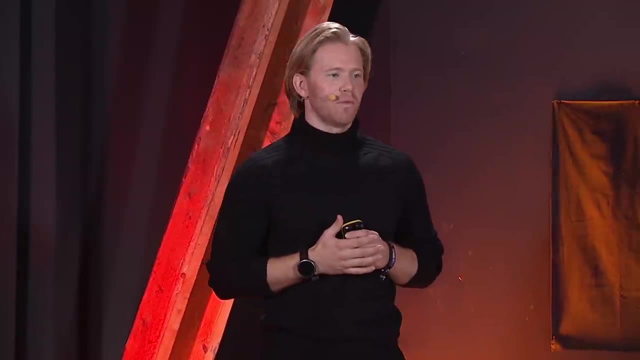 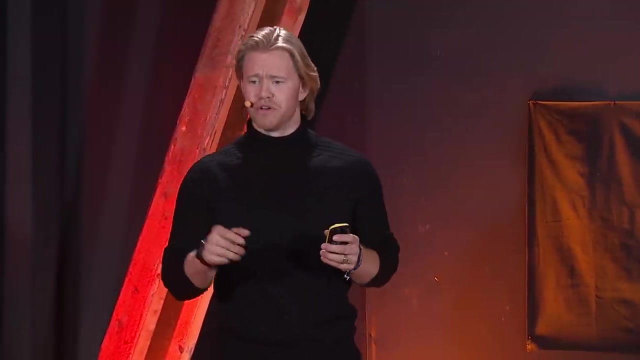 It's a simple action-reaction interaction. Then, with the advent of the microprocessor in the early 1970s, we were able to create programmable interfaces. Suddenly we could choose what button to push or lever to pull and decide what would happen. 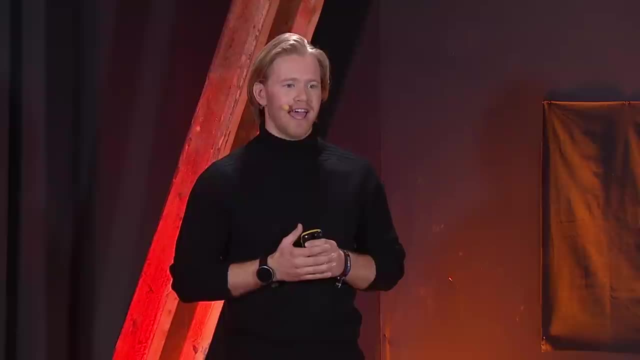 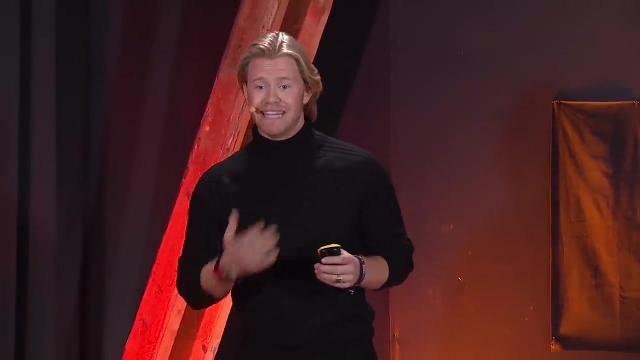 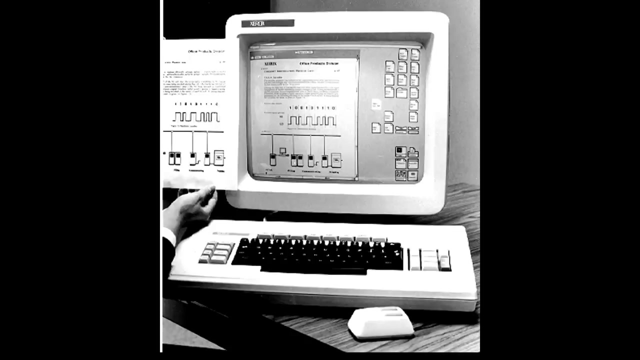 But with great power comes great responsibility, And since then we have had to consciously think about how we create these interactions in order to make them intuitive for us humans. In the 1980s, the graphical user interface was introduced and the mouse and keyboard became the standard on how to interact with machines. 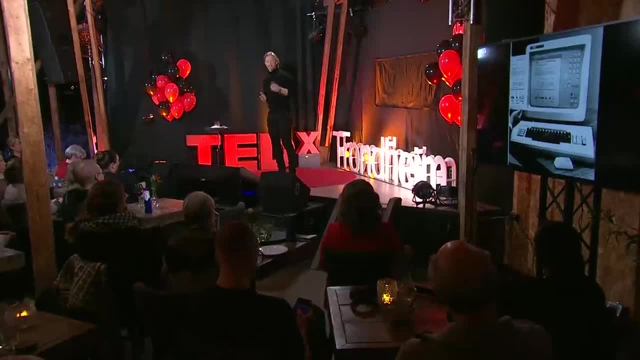 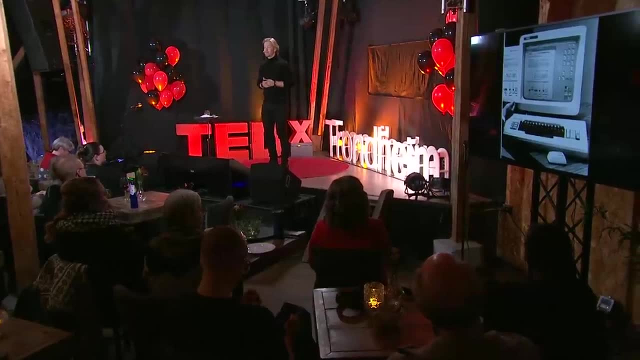 It would take nearly 40 years until this interaction was dethroned by the touchscreen as the most widely adopted one At this point in time. suddenly, anyone would be able to control a machine, and you didn't need to be a programmer to do it. During this time, technology has been rapidly advancing. We have suddenly computers in our pockets with so much excess computational power that it can do more than its core tasks At any given point in time. you have idle processing power, and it's a shame that we don't do more with it. 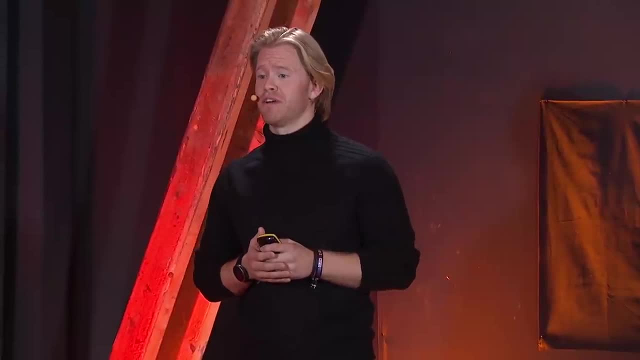 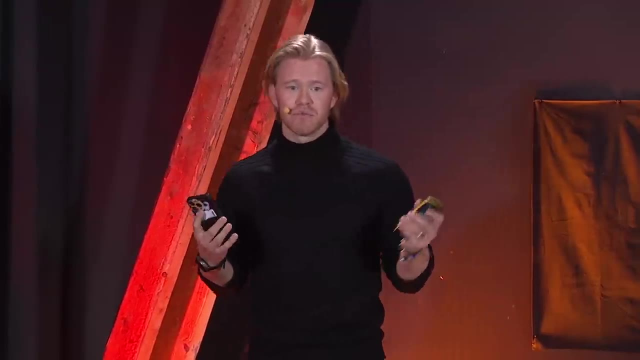 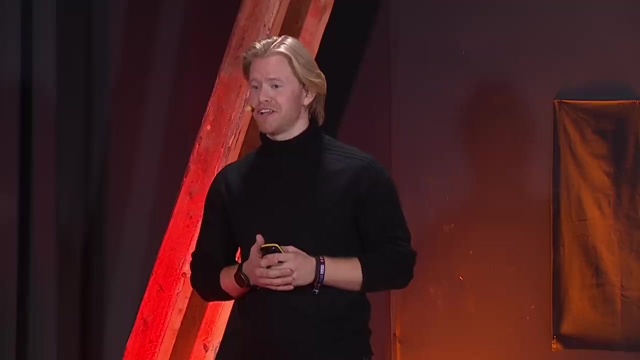 because we could use this processing power to enhance the interaction. In fact, we have more processing power in our pockets than was used for the Apollo missions. So we've come a long way, but there's a long way to go still, Even though we've advanced from analog inputs. 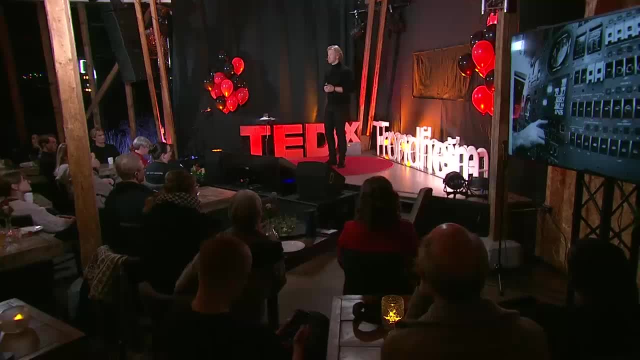 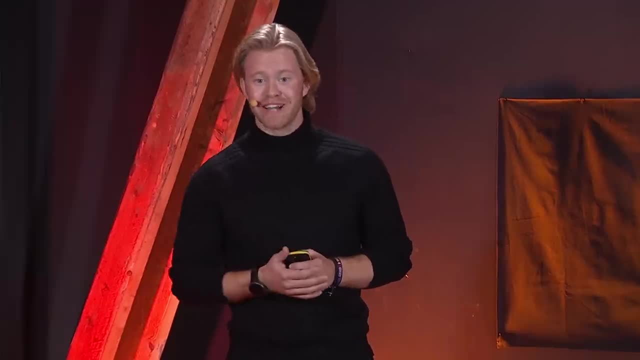 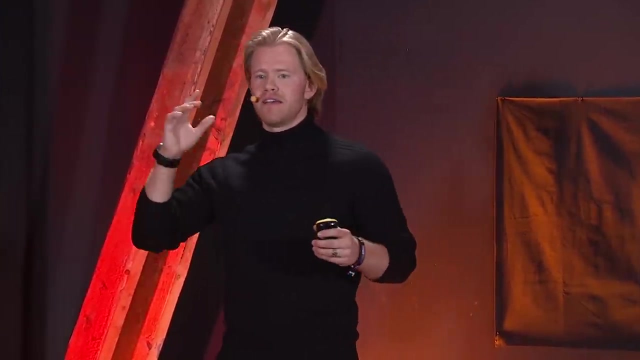 like buttons, and levers into more digital spheres like the touch screens. the paradigm is yet to come. We're now able to equip new machines with sensors, microphones and other means of sensing the environment, and suddenly we could use that as input methods. 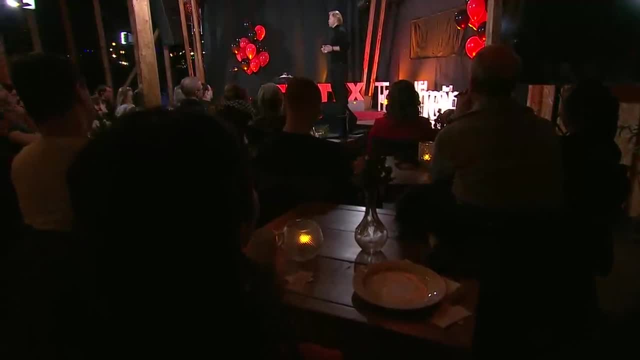 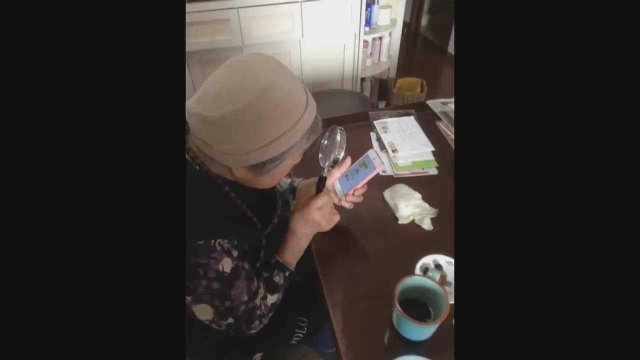 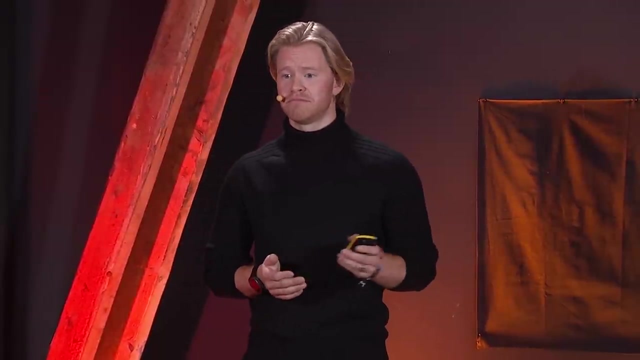 so our bodies could become the control system. There is a digital divide where some people proficient in technology knows how to use all of the gadgets that we now carry around, where some might also be left behind. But we can choose to design a different future. 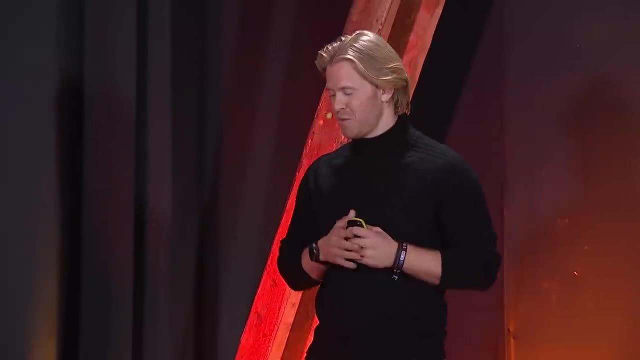 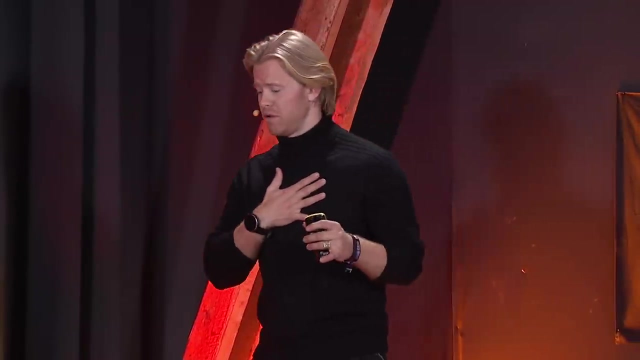 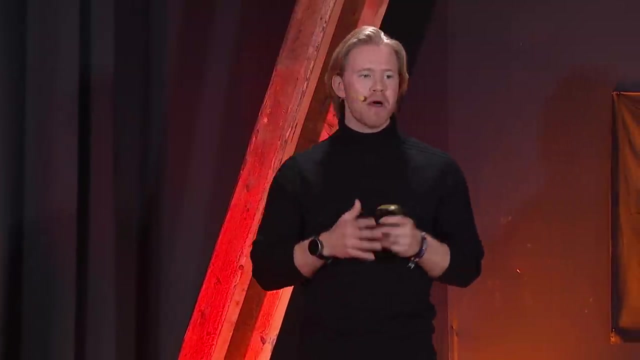 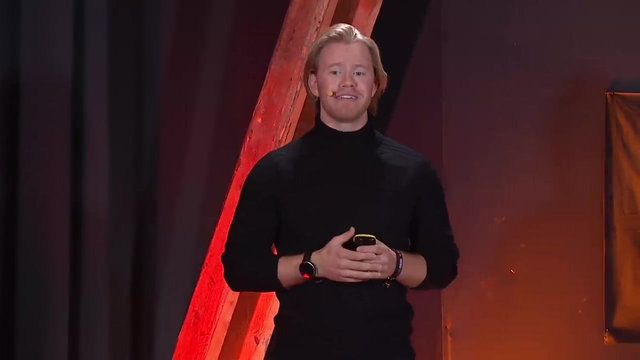 a future that is human-centric, where interaction with machines is easy, effortless and letting people in control. We can create a future where humans experience happiness with positive interactions with their environment, But then we need to make human-machine interaction intuitive, And that is what we have been doing. 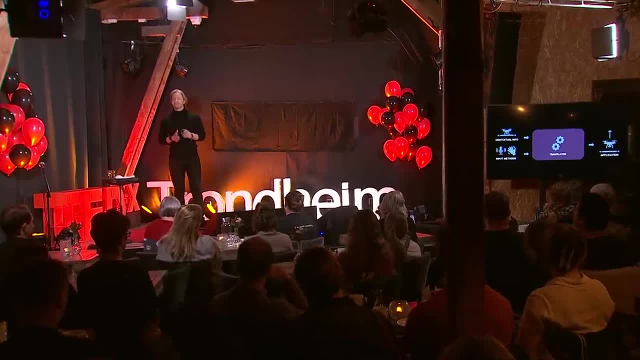 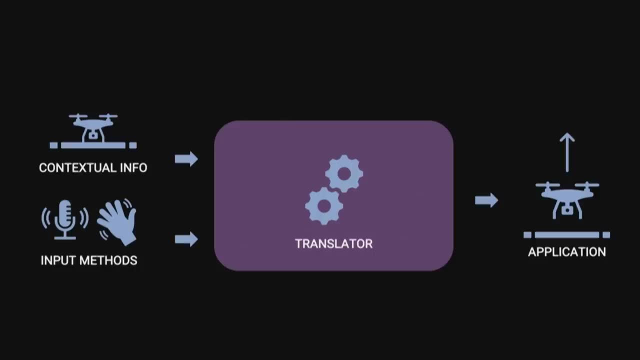 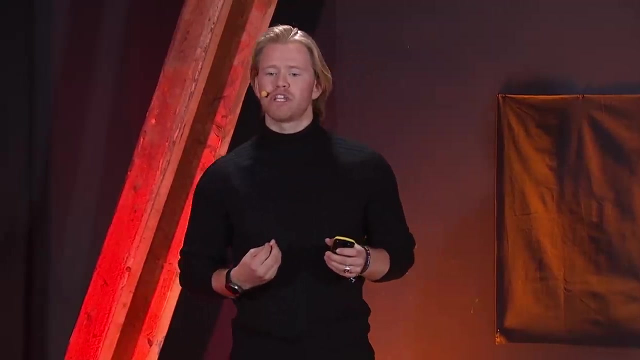 at my company for the past six years. We believe that there is a need for a universal translator that can take into account the environment and the context in which an action is performed, and then analyze the human behavior, try to extract the intention behind that action. 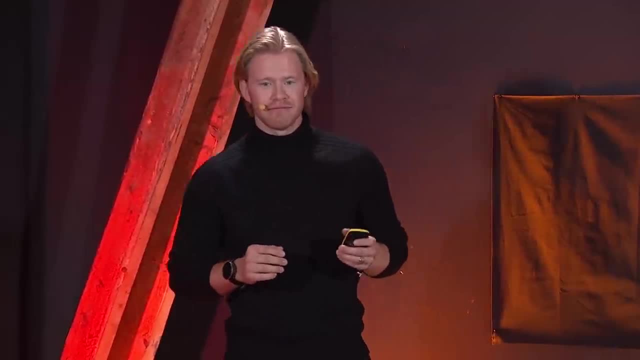 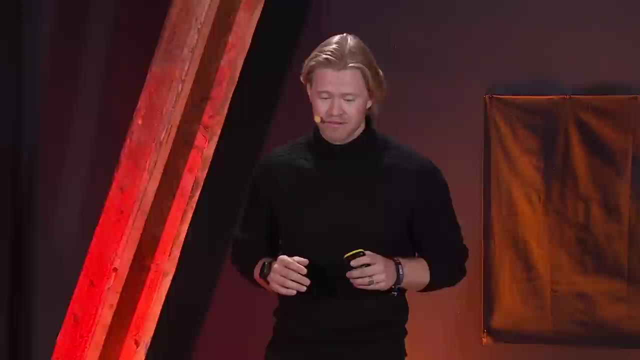 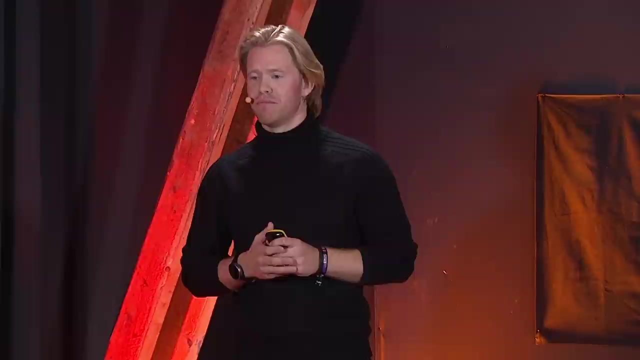 and translate that into machine command. If we manage to do this properly, we could revolutionize the way humans and machines interact. It will become more visible once technology for extended and augmented realities become more mature and usable. We see headsets, glasses. 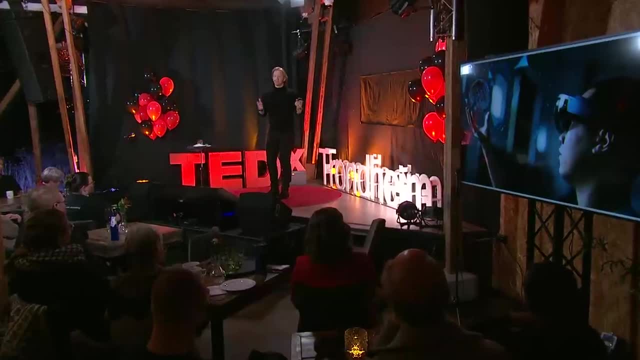 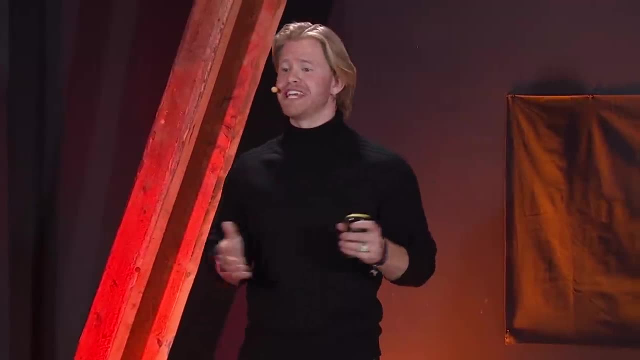 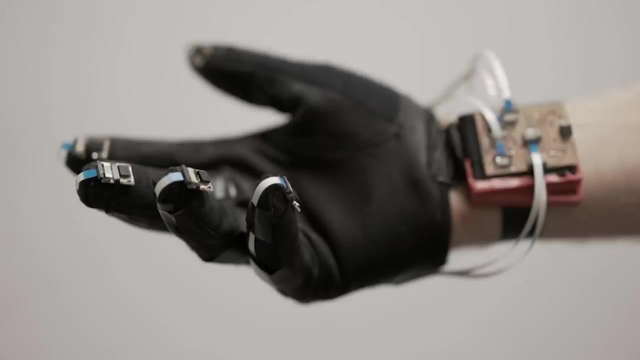 and other means of adding a digital layer on top of our world or merge them all together. My journey into this realm started with a smart glove. It's a sensor-based glove that could control drones. Then it was discovered by Dr Pascal Lee.